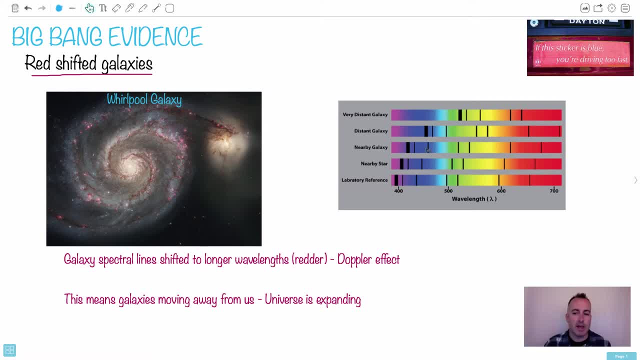 it'll have the same pattern, it'll just be shifted over a little bit. A nearby galaxy might be shifted a bit more, A distant galaxy might be like this. That's what like the Whirlpool is. It's sort of a. 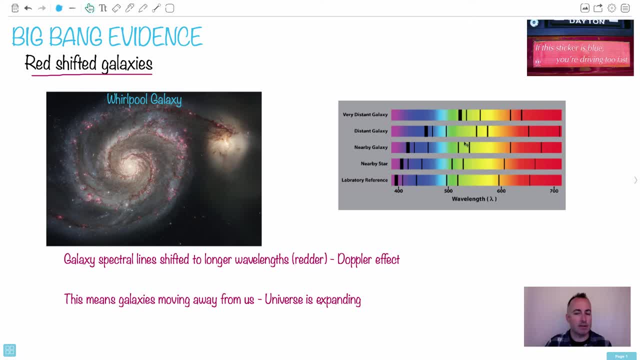 you know, nearby to distant galaxy, something around here? That means things will actually be shifted. Do you notice that? where these spectral lines were found before, let's just compare them here. So we have this spectral line right here. Let's just say like that: 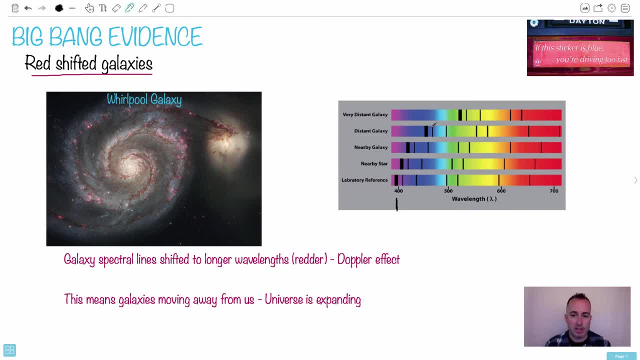 this big, dark, thick band here. Let's just say it went all the way over to here. Do you notice that it went, you know, from here to here. Do you notice that, Like it started here, way up on this distant? 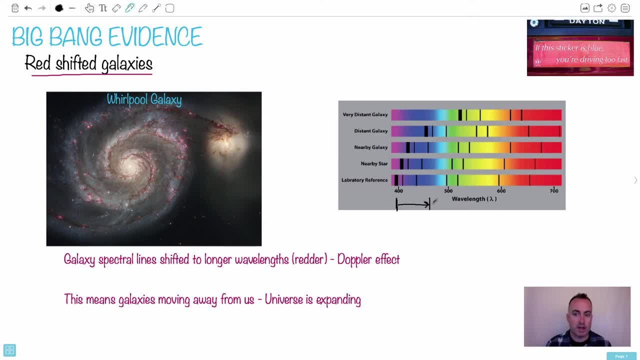 galaxy. it was over here, So look at that. it corresponds to there. Do you see how it's actually been shifted? And it's been shifted to larger wavelengths. That's why we call it red shifted, because larger wavelengths are redder. It doesn't literally mean they become more red. Well, 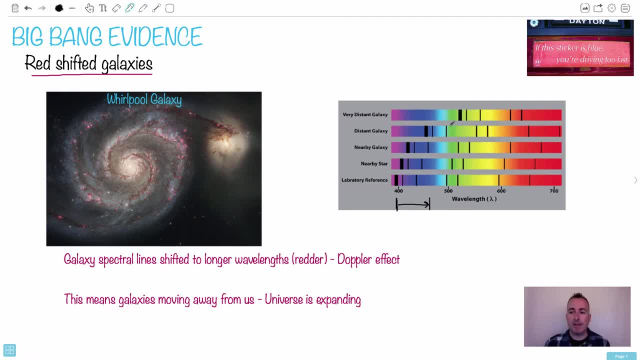 actually there's something called reddening. that happens too, But the very fact that the universe itself is expanding- this is the thinking behind it- is this: If the universe itself is expanding, doesn't it make sense that it would take? you know, let's just assume this is a very simplistic way to draw it, though. 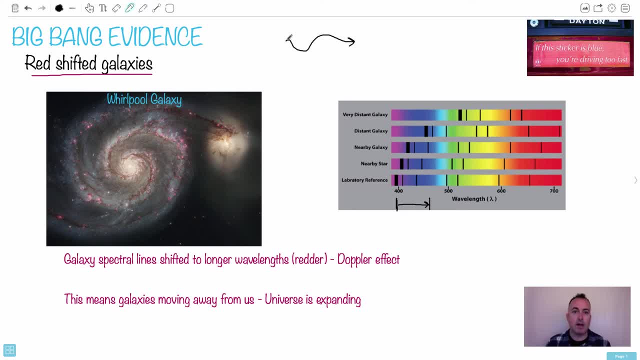 It's not entirely correct but it's, you know it's a good way to think of it. Imagine then you have this sort of wave like this right here. I did a really bad job of that wave. Let me try again. 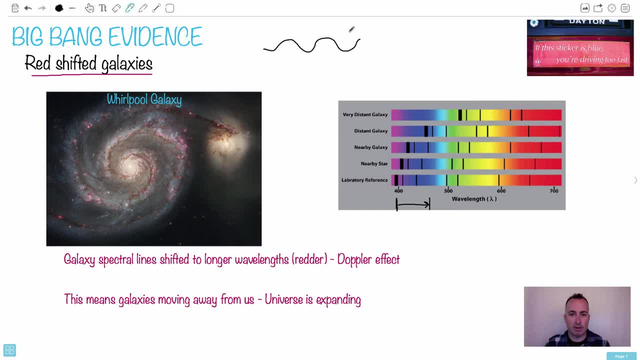 So let's just say, like some sort of wave like this right here, And as the universe expands, what would it do? It would stretch it out. So maybe then it becomes sort of more like this, You know. so just imagine it's like a thing that's just been pulled. If it's been pulled, 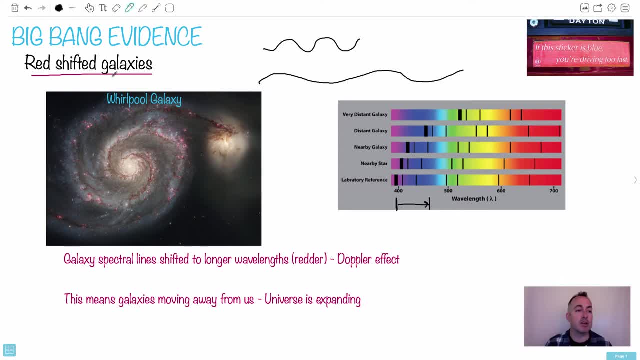 it's a larger wavelength, isn't it? And that's one of the explanations for red shift. Is that? could the? the reason why they could all be shifted towards more red or larger wavelengths is because they're moving away from us. It turns out that's the thing right here, This galaxy. 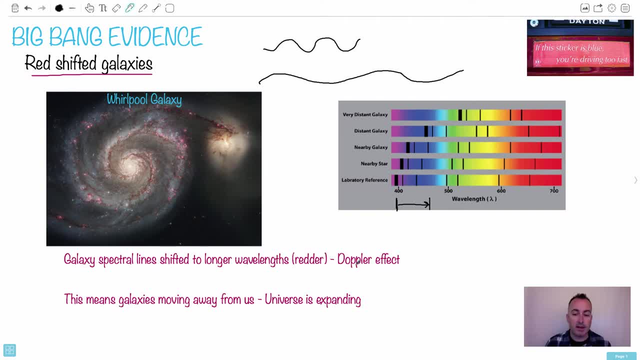 spectral lines are shifted to longer wavelengths so they're redder, And that's explained by the Doppler effect. And this is done. you know, in in the core at least, when we talk about: oh no, it's an HL, but Doppler effect is something that explains that. you know, if something like if a 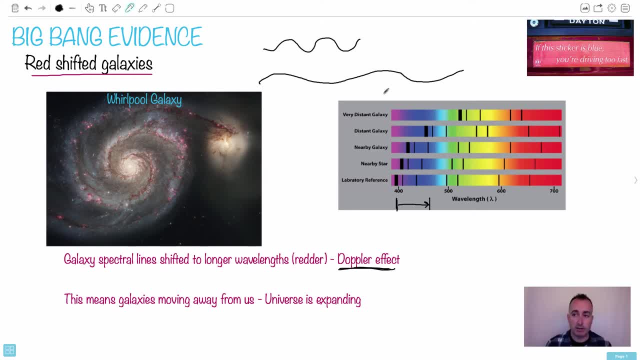 sound is set to higher frequencies. it's a similar idea here. I like this little thing here: If the sticker is blue, you're driving too fast. Why is that? Because blue means blue, shifted means something's coming towards you, Red shifted means it's going away from you. So it turns out when 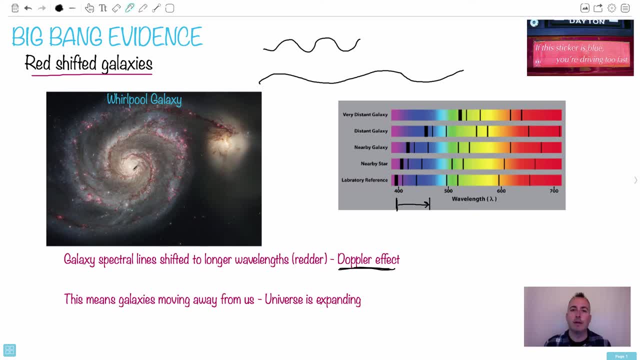 you look at, pretty much every galaxy you can look at, you can see that it's going away from you. So you can look at, they're all red shifted, They're all going away from us, which is really weird. Uh, now there's a few exceptions, There's a few galaxies that are in what we call our local group. 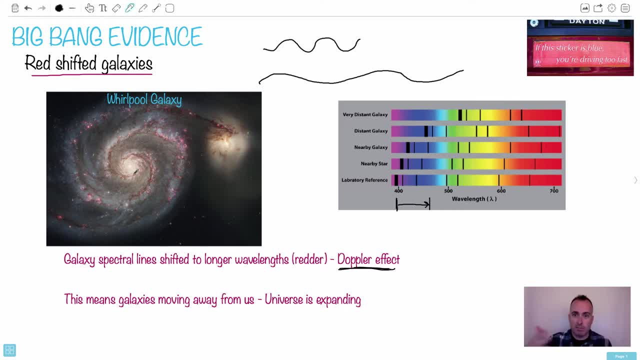 our, our local hood, like Andromeda galaxy. Those would actually be blue shifted. So it's coming towards us. It hopefully makes sense. The close ones are gravitationally attracted to us, but the far ones are more um affected by the universe's expansion. So one of the ideas is that well, 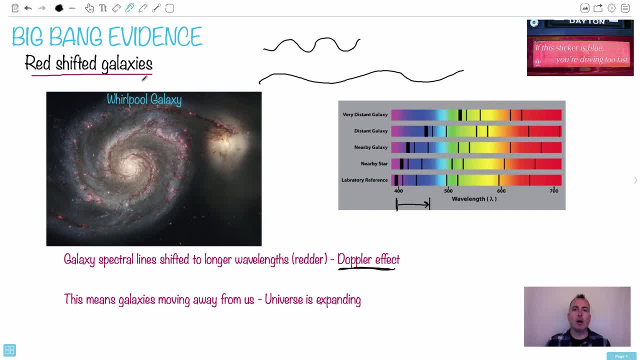 if everything is in a red shifted, that's explained, you know. the idea is that, oh, maybe the universe itself is expanding. That was the idea behind it. right, If everything's going away from us, either we're particularly repulsive or everything is expanding So we. 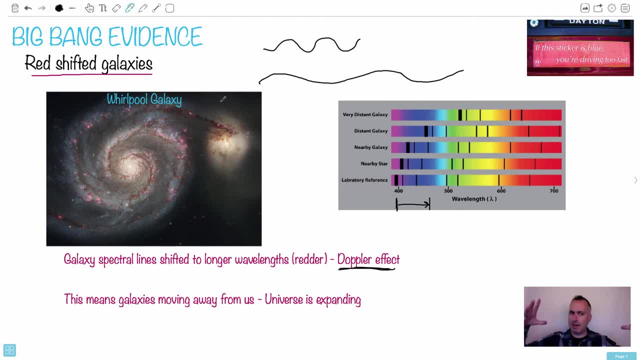 think everything is expanding and then it makes sense. If everything's expanding doesn't it make sense to think about, well then maybe everything was together. So this is one thing. This is one strong piece of evidence for a so-called big bang. So this idea that the universe at some point 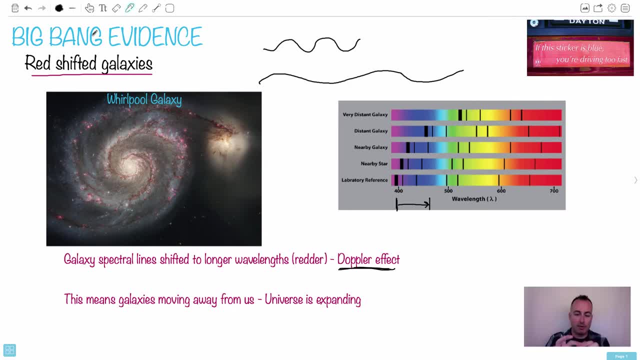 then if it's all expanding, it makes sense that at some point in time there's literally a point and something caused it to blow up and expand. Now, the reason I don't like the theory is because I don't like what it means. but I don't have to like it, I accept it. 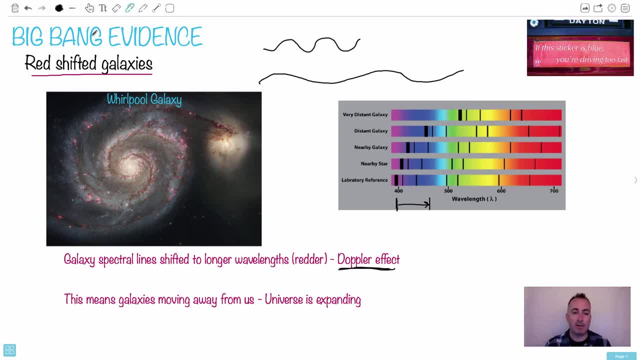 because I have to accept it. I can't think of anything better. So, for example, if you're going to come up with a theory of the universe, it better explain redshifted galaxies, because that we see right. And I don't like what it means because I mean what happened before the big. 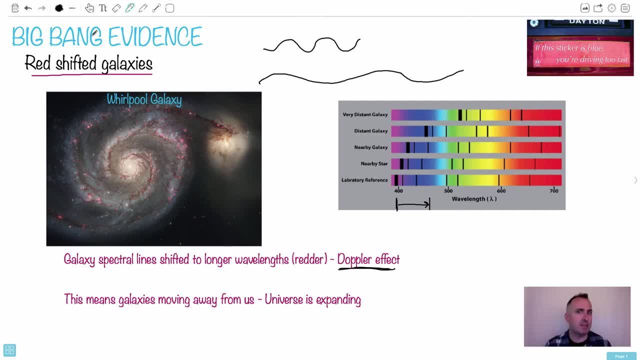 bang. Oh, we don't know. Uh, if the universe is expanding, what's it expanding into? Like my brain has trouble with that, Like don't worry about it, Doesn't make sense, We don't know. Uh, you know. 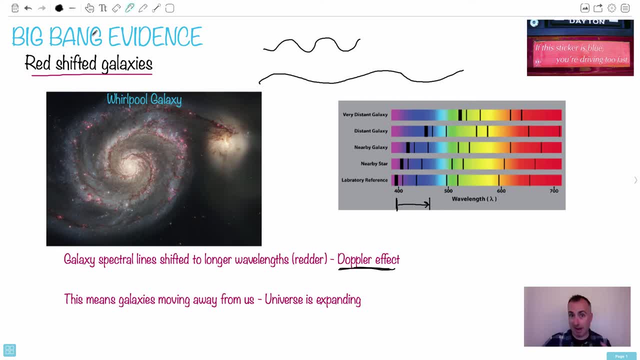 what caused the big bang itself to happen? Oh, we don't know. Have there been other big bangs in the past? Maybe the universe has done some weird things? We don't know, Because the problem is, the only information we can get is from light. Uh, what I think is really interesting about? 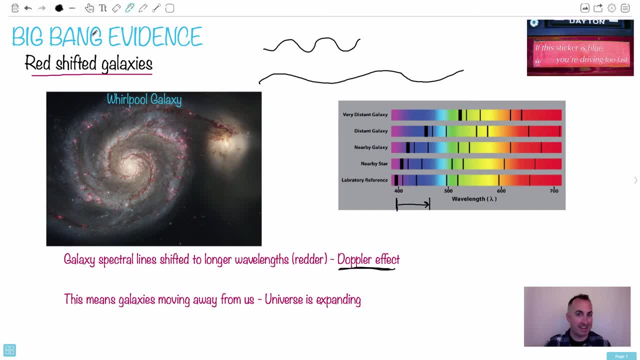 astronomy is this. I mean, the history of the universe is sort of encoded in the light from the stars and galaxies, So we can only tell information about the universe based on what's emitting light. And if it's part of our universe, then it had to happen after the big bang, which means we don't have information of what happened. 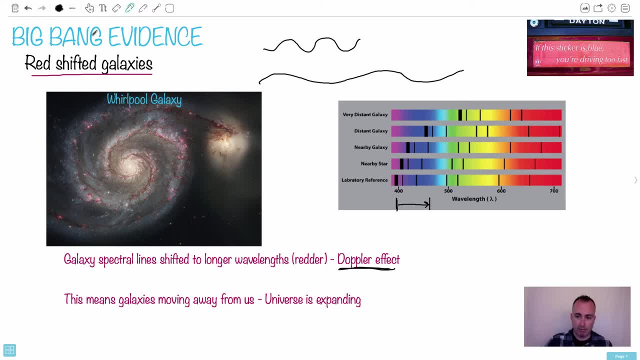 before the big bang. It's just theoretical. The only things we can tell is: you know further away things? We can tell that that happened longer time ago. That's about all we can tell. So we have some limits to this. Turns out we can look at what's the most distant objects we can. 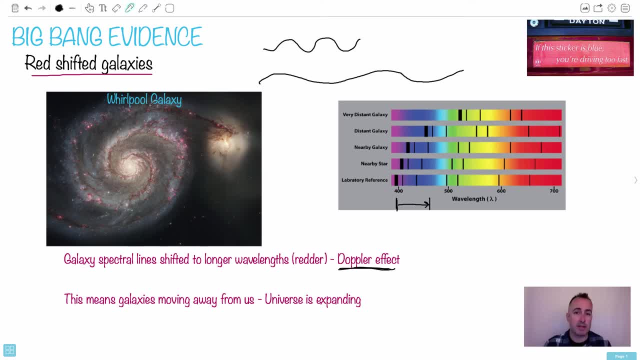 find. Uh, we can also use some different theories, different calculations, and all of them seem to point to the universe is about 13.7 billion years old. It seems to be the age of the universe, So redshifted galaxies are strong evidence for big bang. Even better is this: It's called a cosmic microwave. 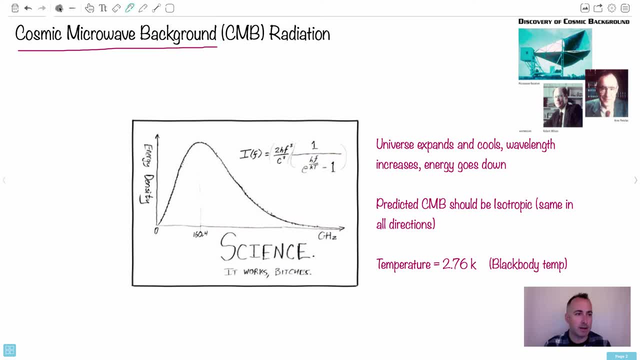 background radiation, or CMB. See what that comes from. So it comes from this area, right? So CMB, So cosmic microwave background radiation. It was predicted that if there was a big bang like this and the universe was expanding, it should cool, Um and so because of this, and they could figure. 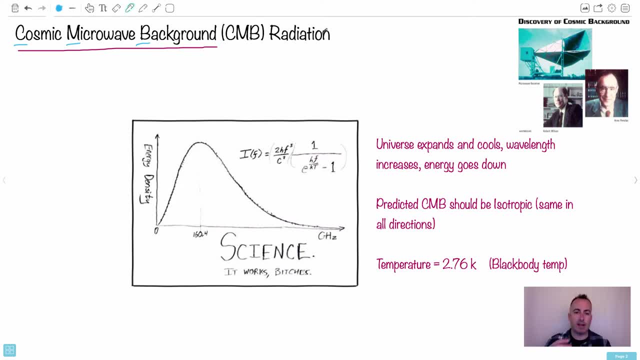 out the, essentially the um. well, because the wavelength, you know, larger, the wavelength will go down. Uh, sorry, Uh, we'll go up, Sorry. And that means the energy should go down because equals HF, If you remember that equation: equals HF, which is: 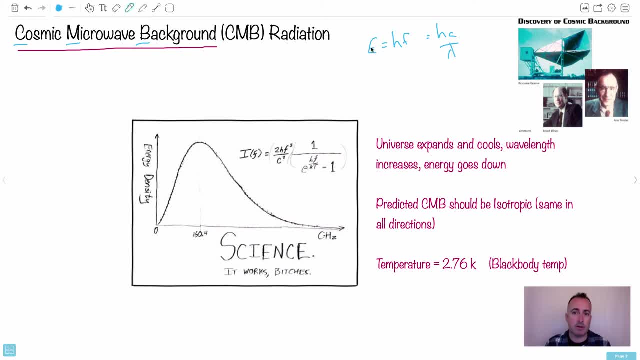 HC over Lambda. So if the wavelength gets bigger, the energy right here gets smaller. So they could actually predict- they mean some very clever astronomers, They could figure out, uh- what this radiation should look like now. So if it happened 13.7 billion years ago, what should? 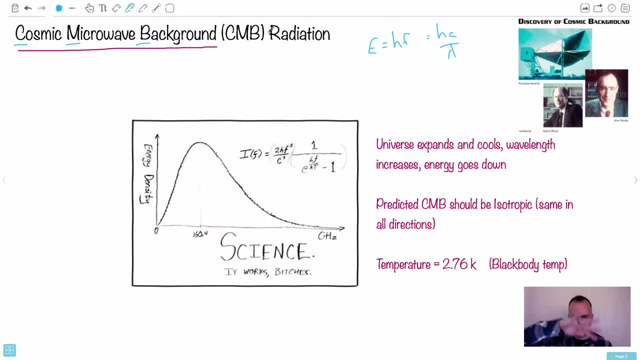 their radiation be like now. And it wasn't just one value, Remember, it's this whole spread of data So they could figure out basically what. should it be The peak uh wavelength? Remember we have this other equation that the uh wavelength times the temperature is equal. 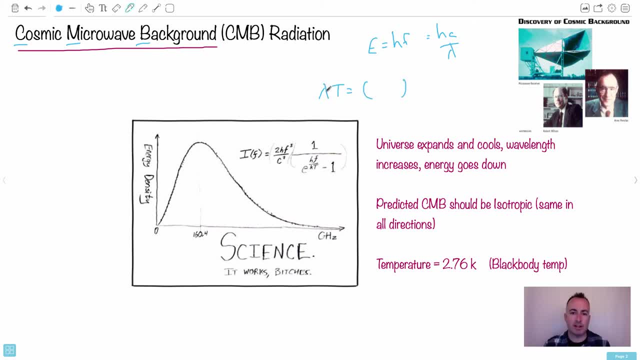 to some constant uh, which means basically that wavelength and temperature are kind of related. So if you can know they could figure out basically the temperature of this cause, they could figure out the wavelength that should be remaining, you know, after it's been. 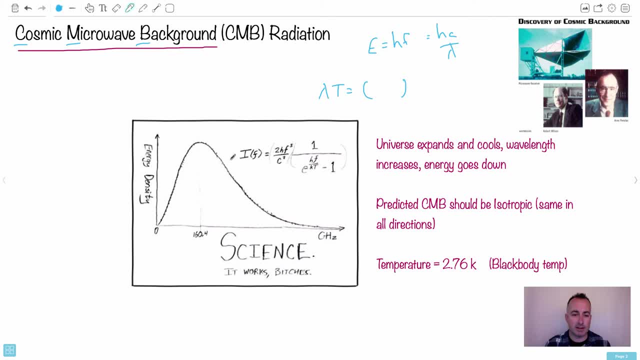 stretched out and it turns out they could calculate all this and you can get an equation. It looks like this: look, there's an exponential here. Now, you don't have to know this for the um astrophysics option itself, but uh, and I'm sorry about this, Some people might get offended. 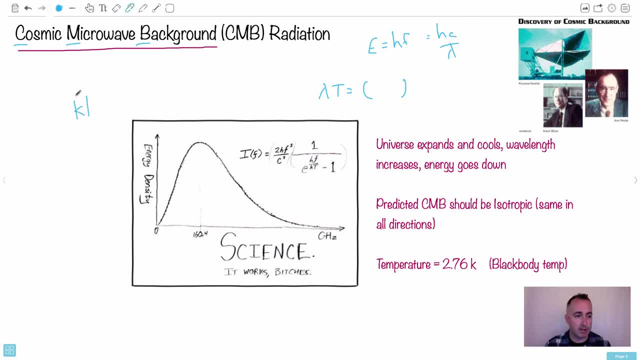 by this, but actually it was done by a guy in a random Monroe. Uh, his website is called oops, called X, K, C, D, It's brilliant website, Uh, and one of the things he did is that science it works. bitches, not literally right, Just like an expression. Uh, don't want anyone to. 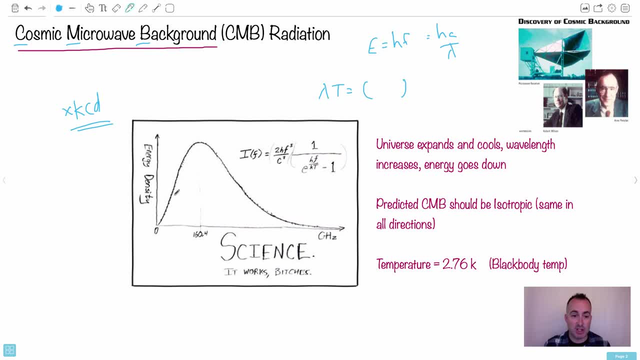 get offended here, But, um, what happened is this? they could predict, then, the shape of this whole uh data here, And I hear they've done it in frequencies, but that can be done in wavelengths, It can also be done in temperature. Just keep in mind. So frequency, wavelength and temperature. 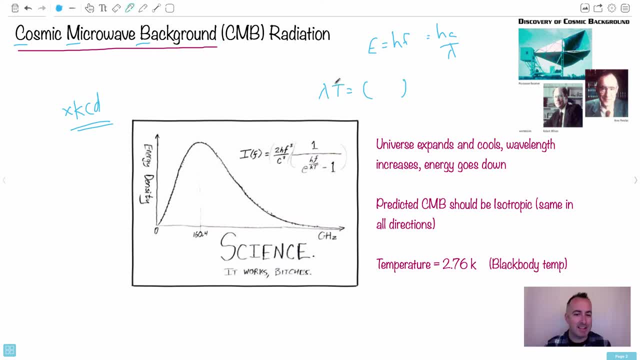 although they're not the same, they sort of relate to each other And basically they predicted that there should be a peak sort of a wavelength, a peak wavelength that corresponds to a temperature of 2.76 Kelvin. That should be the sort of black body temperature of the overall universe. It 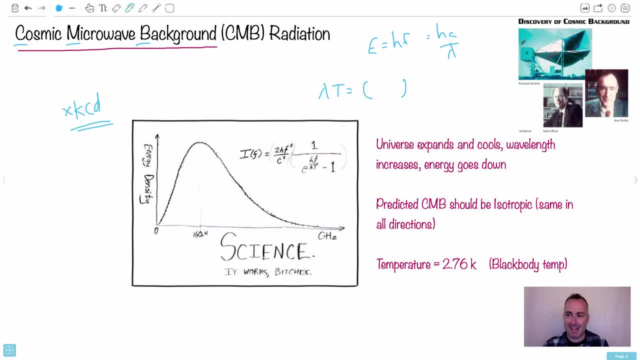 should be pervasive. What's kind of fun is that? um a little while later, there's two guys named Penzias and Wilson. They were looking at- uh, the night sky- for totally different reasons, but everywhere they looked with their fancy new. 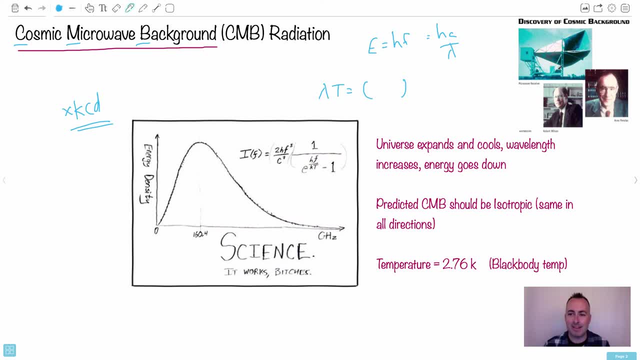 telescope here. uh, they could, they could catch this extra signal. It was pervasive, It didn't matter where they looked, It was always the same. Uh, so it turns out then, if you do that data, what he's done here, he's drawn here, See this, this, uh curve that corresponds to 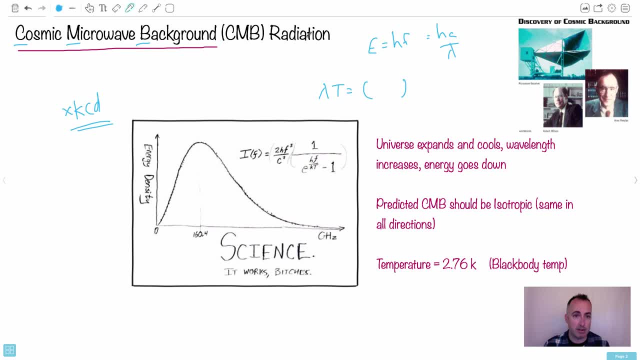 that equation that was predicted from, uh, basically from CMB. So they predicted math, that there should be a shape that should look like this. Now what's interesting is interlaced on it. See these dots here. Those are the data points that these guys found, So it's one of those. 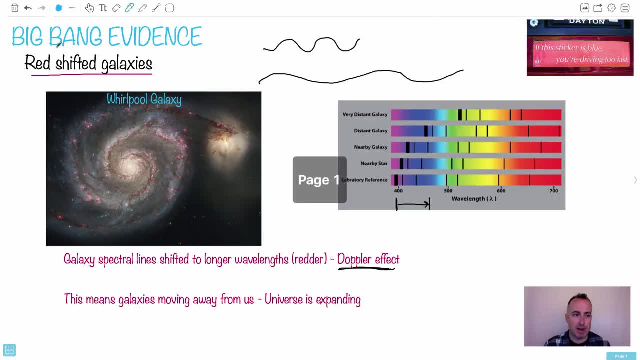 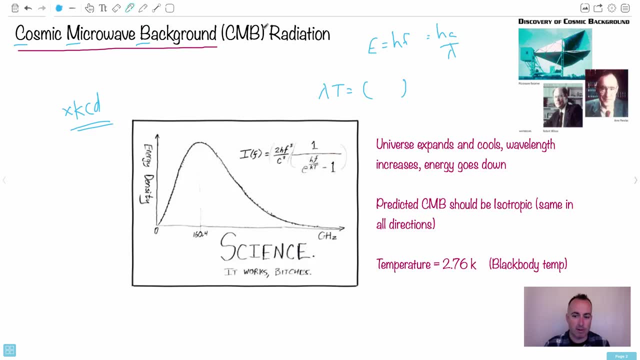 examples where. remember, in science, not only did this big bang theory explain existing things, it predicted the existence of a pervasive cosmic microwave background that should correspond to a temperature of 2.76.. In fact, they could map out all the different data points that it should do. 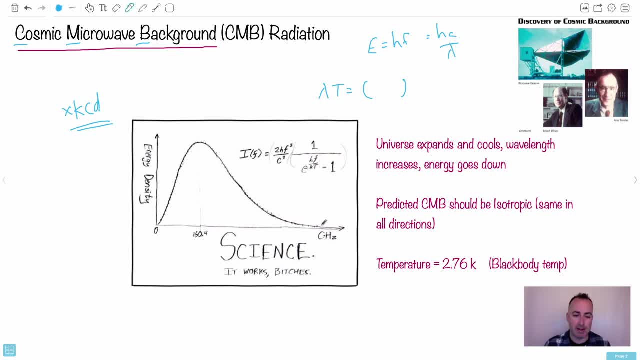 And in real life all of it matches and it matches exactly, which is awesome. That's why he was excited and said: science, it works, bitches. Uh. so it says the universe expands and cools, wavelength increases, So the energy goes down. Predicted one should be isotropic. And what does that mean? It means no. 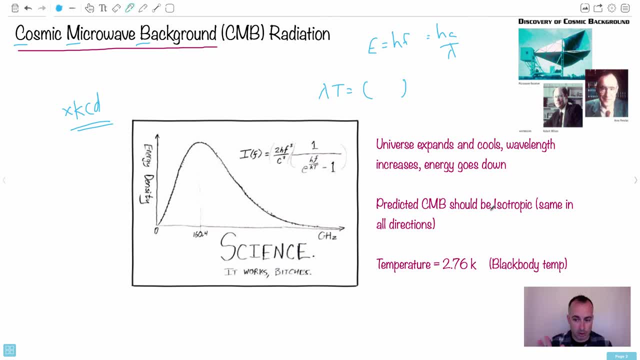 matter which direction you look, it should be the same. It should be the same, By the way, I forgot to put it. It should also be- uh, whoops, should also be homogenous. Homogenous means actually literally the same everywhere. 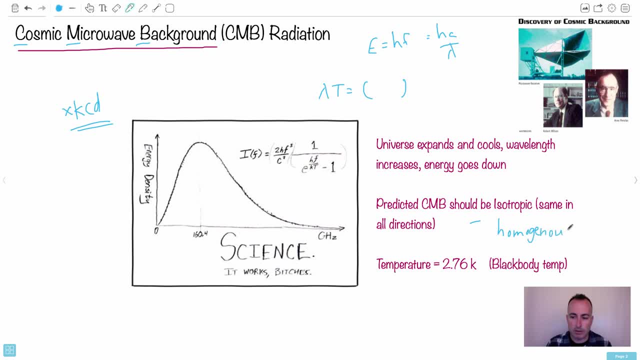 Like in the same, in like space, homogenous also should be homogenous, should be isotropic and should have a peak wavelength of 2.76 Kelvin. So that's why, although I don't like the theory of big bang, I accept it fully because, come on, this is a really pretty strong evidence. No one's come. 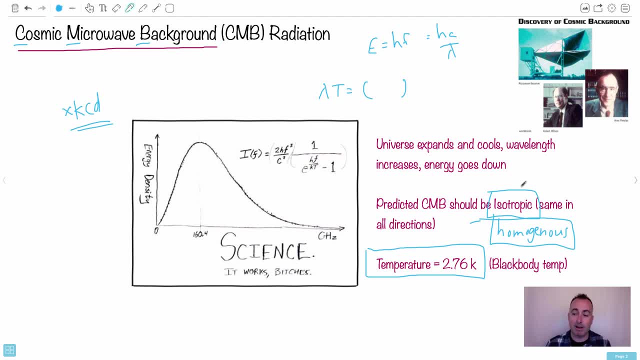 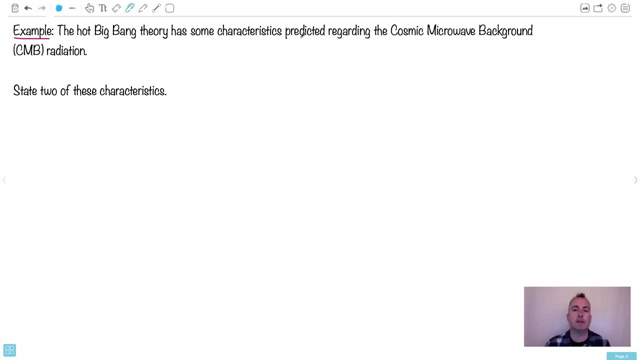 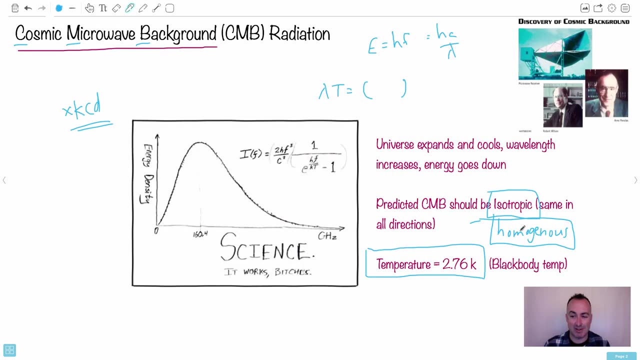 up with anything better than this? Well, people would argue they have, but this is by far the winning one, Um to use an example from an exam question. So the hot big bang theory has some characteristics predicted regarding the MB state. two of these characteristics? Well, we could state any of these three: isotropic: 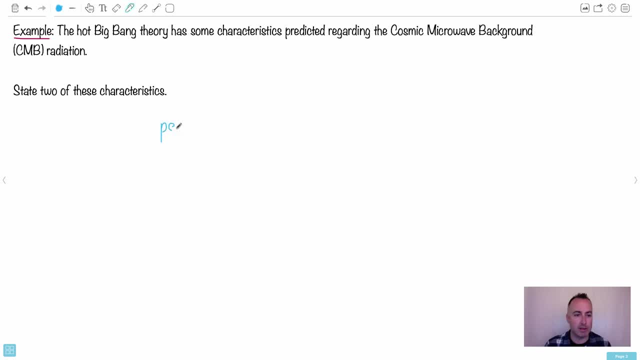 homogenous, or temperature. So maybe we could say that. So we could say peak temperature, Remember, cause that's the wavelength here, That's a Lambda max corresponding to a temperature of 2.76 degrees Kelvin. That could be one of them. I mean, if you're supposed to do two, you could do that. 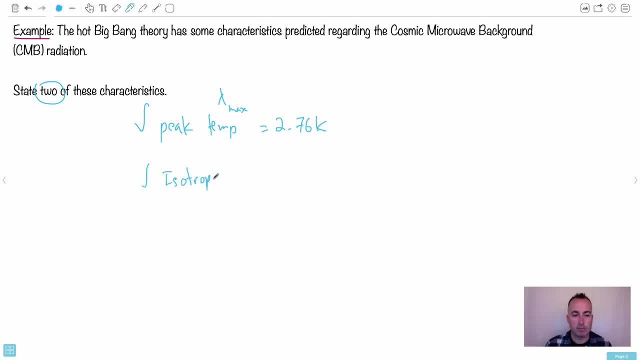 You could do isotropic, which means same in all directions, or you could say homogenous, right? Any of these two would work. So in that sense it's pretty easy, right? It's not that hard. So the questions they're going to ask you are fairly straightforward, but what they mean is super deep. and actually really interesting.